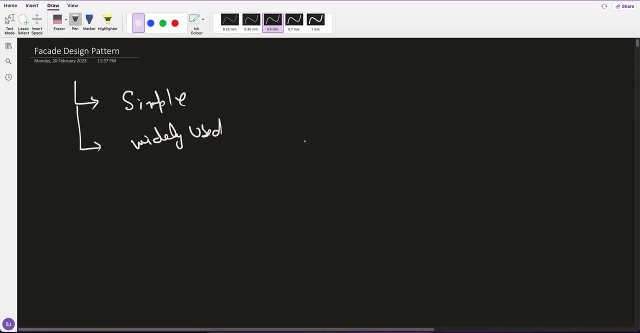 Right. So before going this, I will tell you what we will cover today. So I will cover facade design pattern. I will tell you different real world use cases. Plus, at the later part of the video I will tell you about facade versus proxy pattern. Also, facade versus adapter pattern. 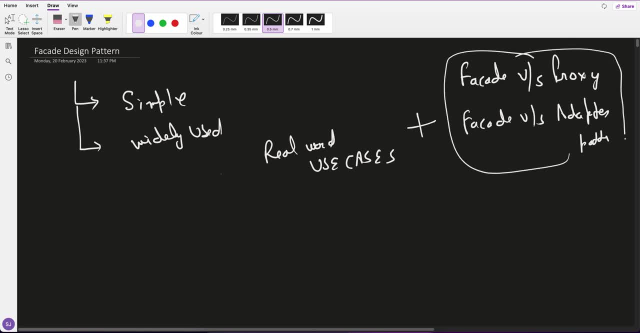 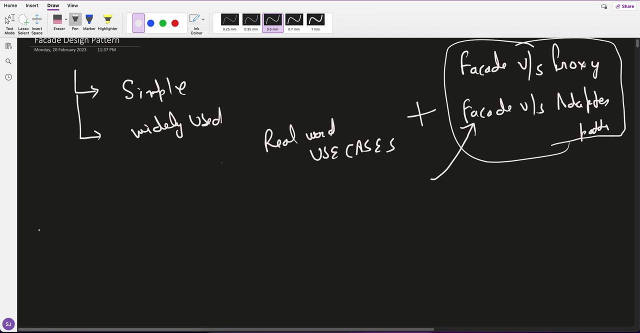 Because they are little bit similar and many candidates got confused between this Right. So with I will show you different scenarios: where can we can use facade with different, different examples, And I hope it will help you to differentiate. okay, where to use facade, when to use facade- Okay, so let's start. Okay, let's start with facade. So what is when to use it? 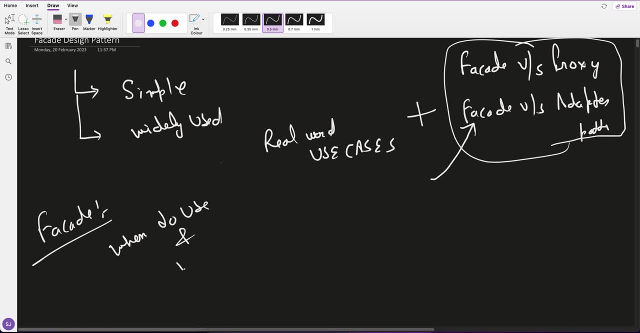 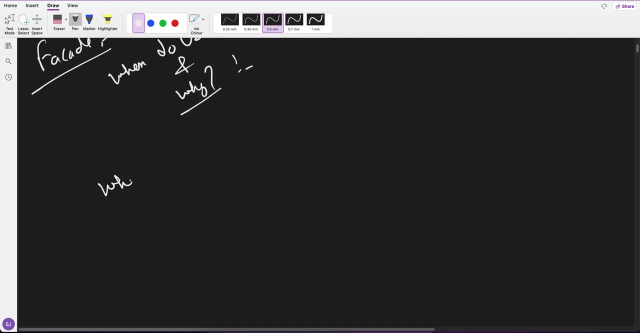 When to use it. When and why? So facade is used when we have to hide the system complexity from the client, That's all. So when to use facade, Just always remember this: when and why: whenever we have to hide the system complexity from the client, then we have to go for facade. 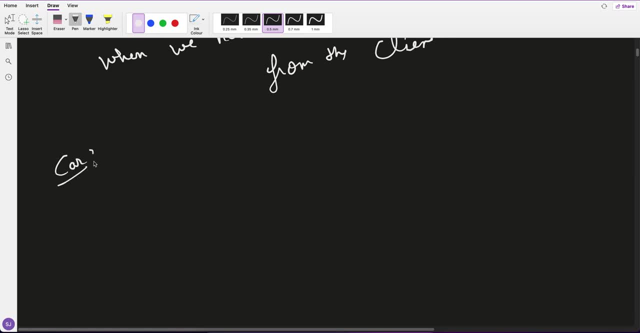 for example, car, ok, so we all know that whenever. so let's say, you are a client, so as a user, user, we who are driving the car, we are a client. so user know that when he press, or when he press accelerate method, accelerate function, what will happen? a speed goes up and when 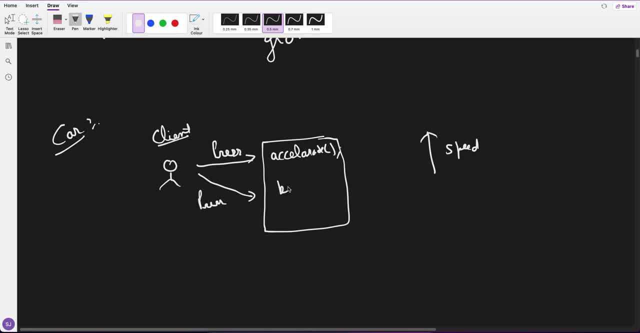 the user press brake, what will happen? speed goes down right. so that's how, as a client, we know the functionality: if i click, if i press accelerate pedal speed will go up, and if i push the brake pedal speed will go down. but the real complexity, the system complexity. 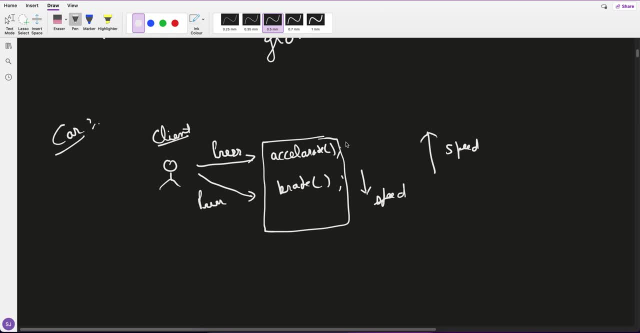 behind the accelerate does clients knows it? no. so when actual this method got called right may be internally a system has so many classes which are interacting with each other to actually make the speed up right client i do not bother like how actually the speed is getting increased. ok, this engine. 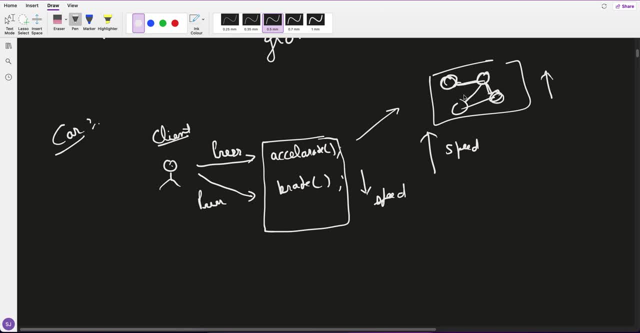 is interacting with gear. gear is interacting with this. we don't know right. we are less bothered about how different components of a car interact together so that speed goes up. we don't care. all we know, all we care about is if we press the accelerator pedal speed. 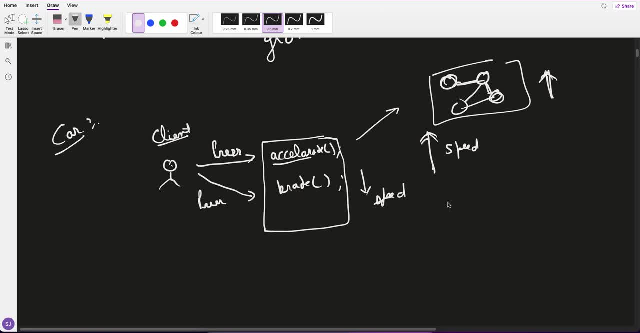 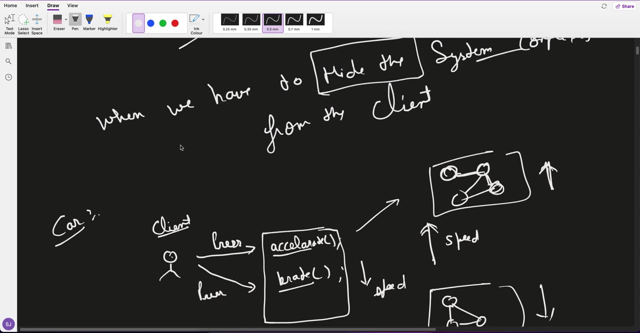 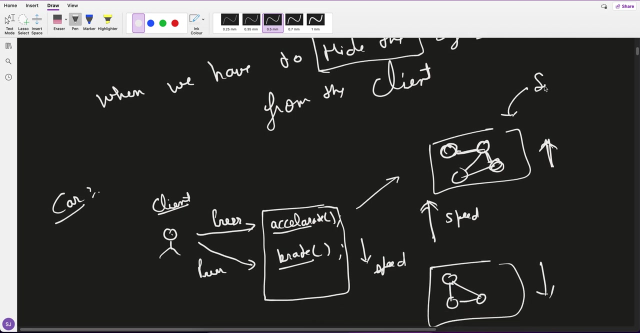 should go up. we all care about if we call brake speed should go down. so if we go with this definition, so now what we have done is we have to hide the system complexity. so this is our system, right, and it is very complicated system. let's say there are thousand of component in a car which 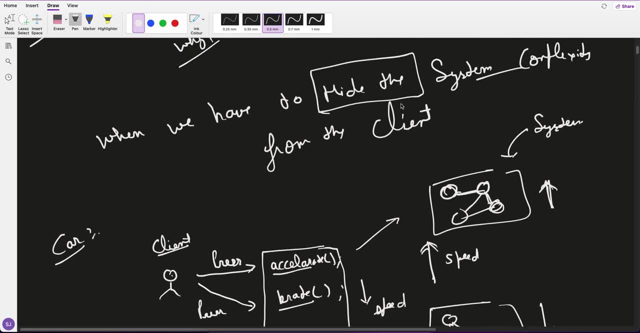 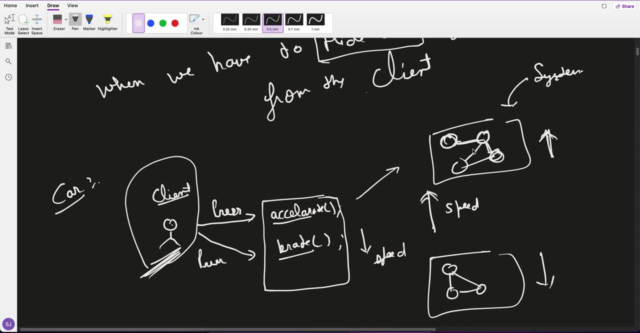 are interacting with each other, right? so we have to hide this complexity, right? so we have to hide this complexity from the client and we have to hide this from the client. client should not know about the thousand components, how they are interacting, right? so he is all interested in acceleration. 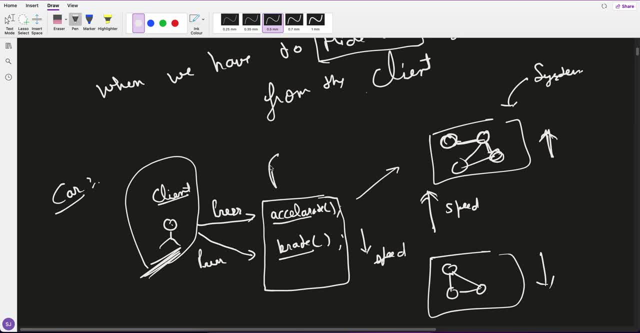 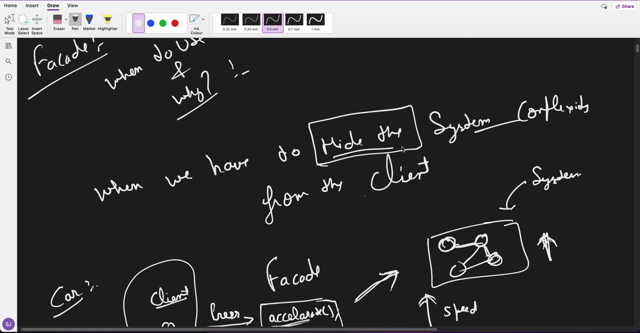 brake and other functionality, right, so this is nothing but a facade layer. if it is not much clear as of now, don't worry, i will tell you many more examples. it will get very, very much clear. but currently only remember that when to use facade, whenever we want to hide. 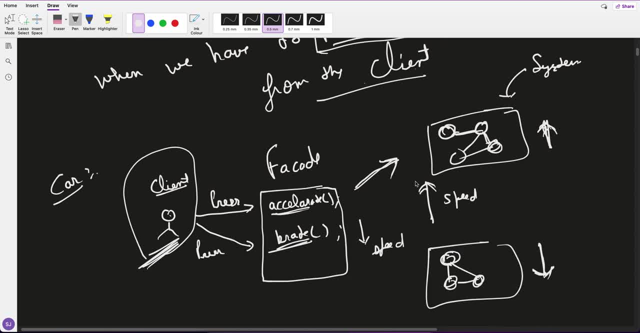 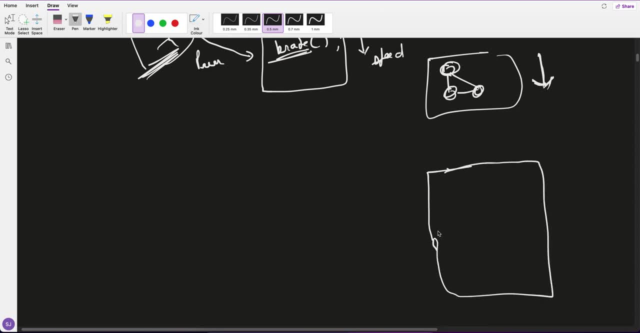 the system, complexity from the client, right. so with this example at least, you know that there is a system which has many components or many classes. you can say that many classes- class 1, class 2, class 3, class 4 or let's say class 100 something- and they are interacting with each other. so it's a very complex system. 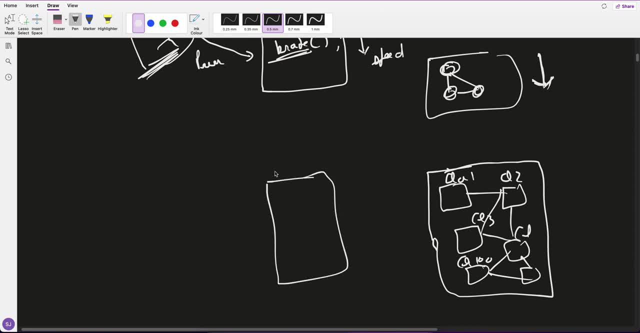 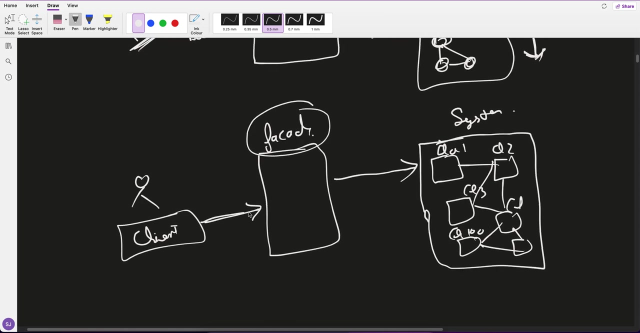 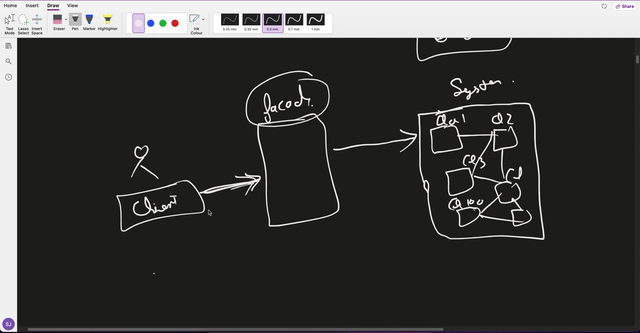 right, so facade is just a this layer, right, and this is actually the client. so client interact with facade and facade internally interact with the system. right, so this is what known as facade. but always remember that we are not forcing client to always talk with facade, right? client if wanted. if client wanted. 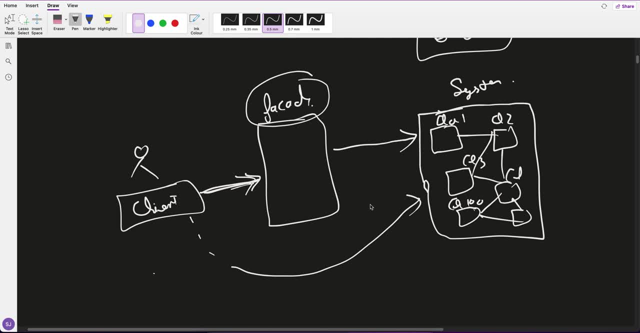 client can also talk directly with system right. if client wanted, client can also talk directly with system right. so facade is not a mandatory. first of all, we have to always remember that we should not enforce client to use facade if he, if client, wanted to use any of the class, so let's. 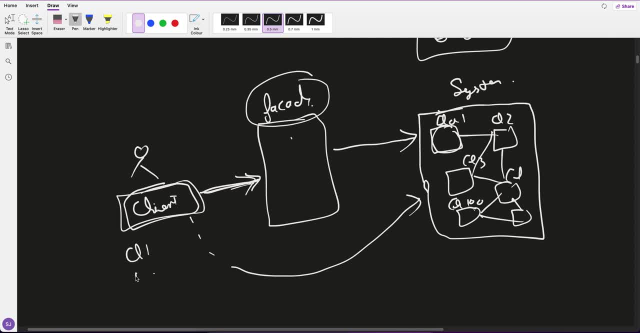 say facade, client say that okay, no, I want to use class 1, class 2, class 3. so we should not force client to use facade to do that. so it client is independent. like if I want to use, client should be able to use the components independently and whatever the facade logic. 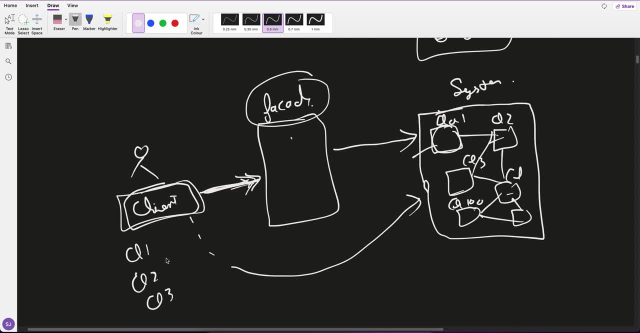 client say that, okay, I can build that logic into mine. it should be open so. but it's client choice that, whether they want to build a complex by themselves or better way is that we can create a facade layer and client can interact with that right. so all the complexity and 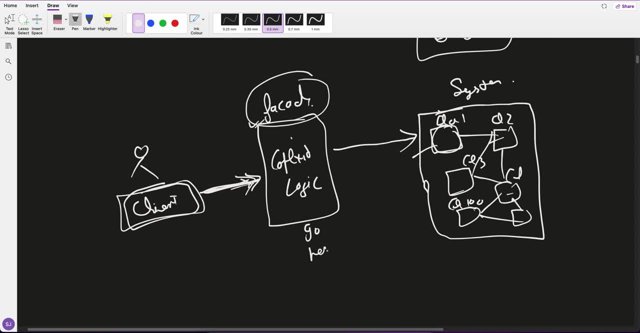 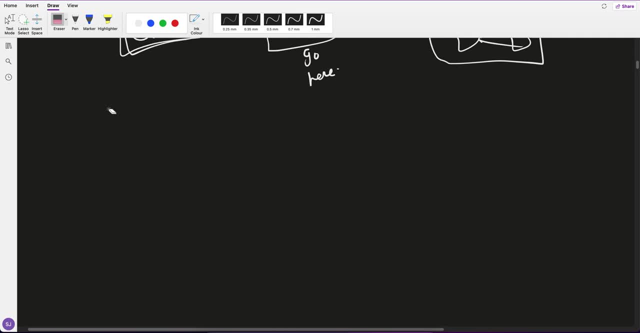 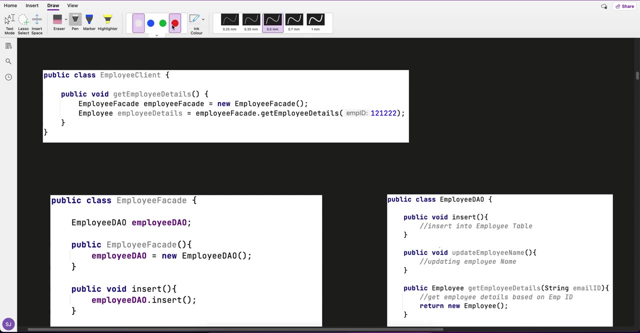 logic goes here. so all client has to do is just call the facade. so till now it is clear, simple. now let me tell you the different scenarios where we can use it. scenario one: right, the example, the car example which I gave you. right, it's very much similar to it. so here I have. 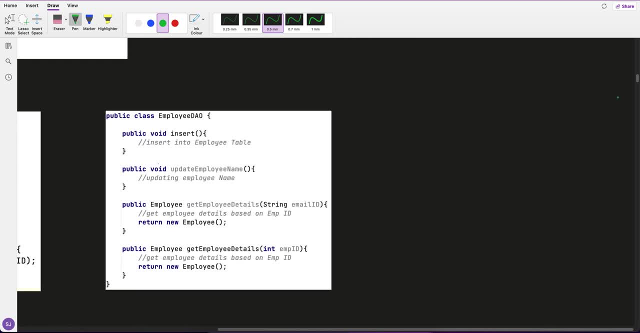 created an employee Dow, employee Dow and. and those who don't know what is Dow, Dow is right. I have created a class called data access object, so a class which interact with DB: insert, update, select, all method goes here and actually it interact with the DB and insert the root. 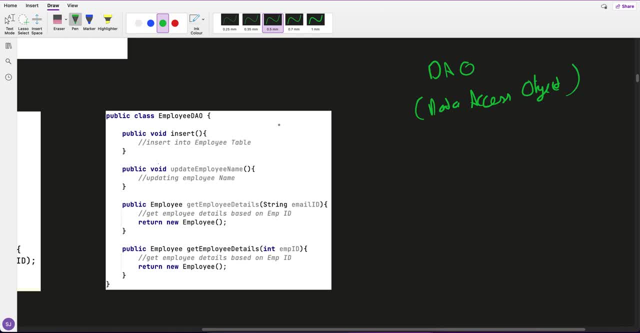 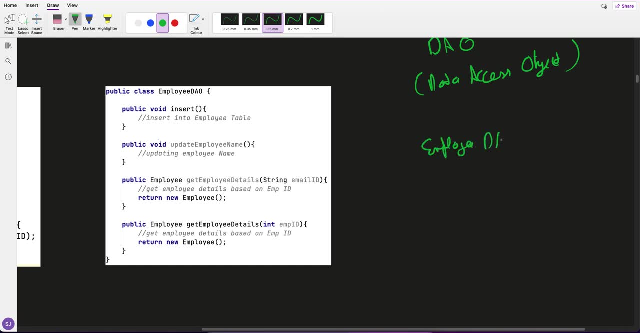 get the row, update the row. so that's where we call this Dow. okay, so now I have created one employee Dow, and this employee Dow can have many methods. Let's say insert, update or update employee name, update employee address. right, then it has. get employee detail by employee ID. get employee detail by email ID: email ID: similarly. 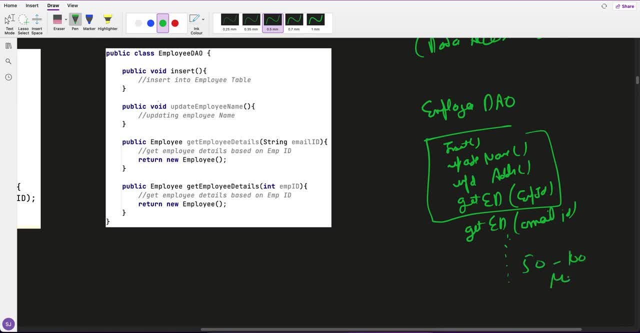 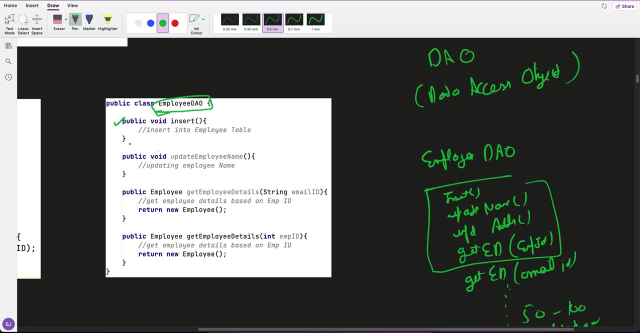 let's say there could be 50 or 100 methods, right. there could be so many methods, right. so I have created an employee Dow, and I have put method like: insert: update employee name, get employee detail by email ID, get employee detail by employee ID, and there could be many. 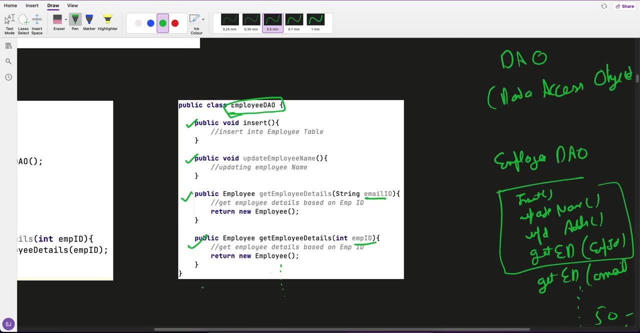 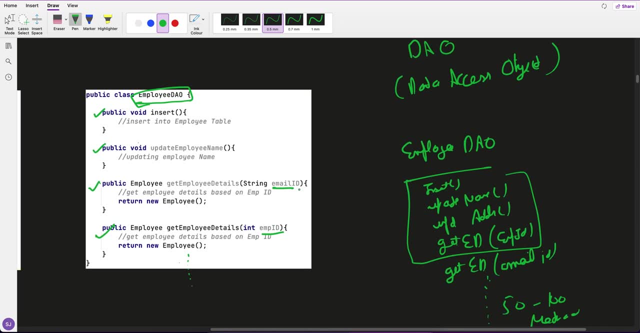 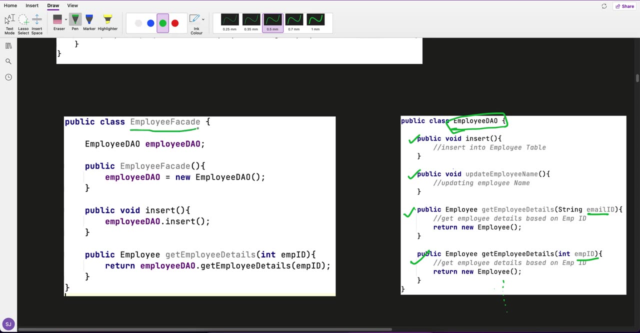 more methods. but let's say our client is only interested in insert and get employee detail. it doesn't bother about all the 50 or 100 methods. so what we can do is one way is I am creating a facade here, employee facade right, and in the employee facade what methods? 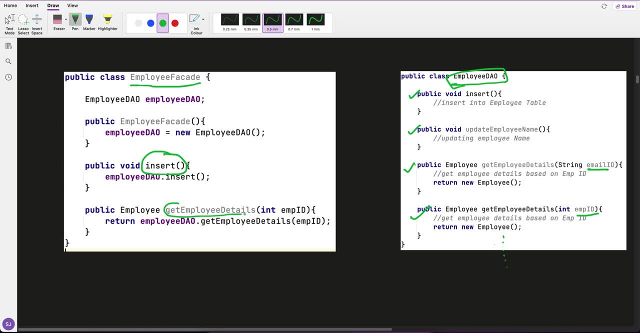 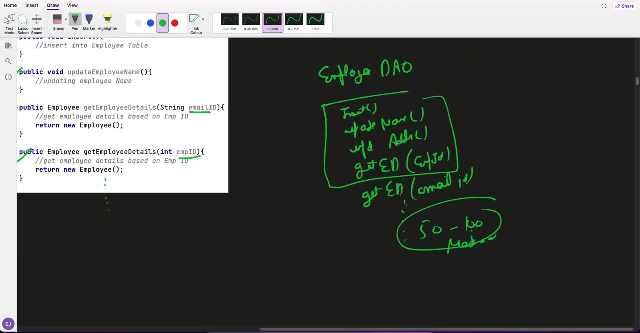 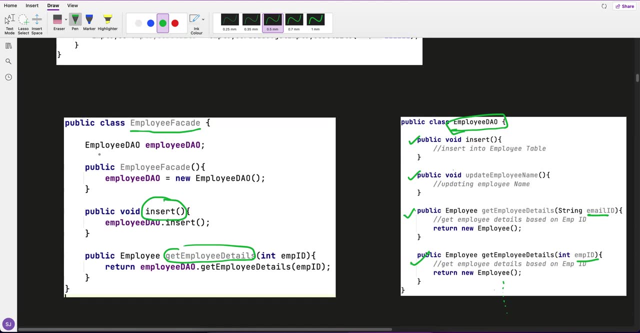 I have exposed, insert and get employee detail via employee ID. so client is only bothered about this too. it doesn't bother about what all other 50 or 100 methods involved, right? so here, if you see in the employee facade it has employed Dow object. so employee facade. 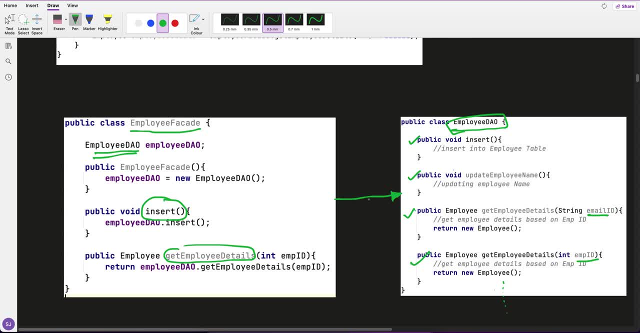 has Employee Dow right, so it creates. so now you know one more thing: that the facade takes the responsibility of creation of an object, of all the components that interact with. so currently it is interacting with Dow, so it takes the responsibility of initializing its object also, and it exposed only those method which client required it. so this is my client. 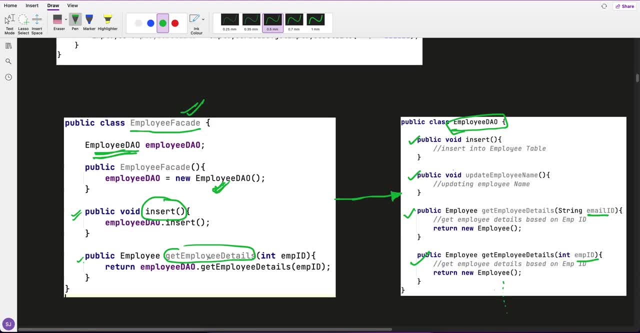 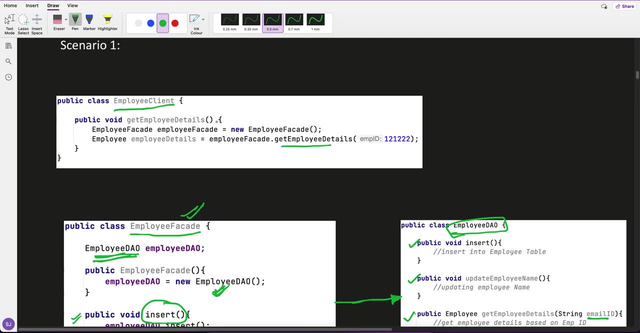 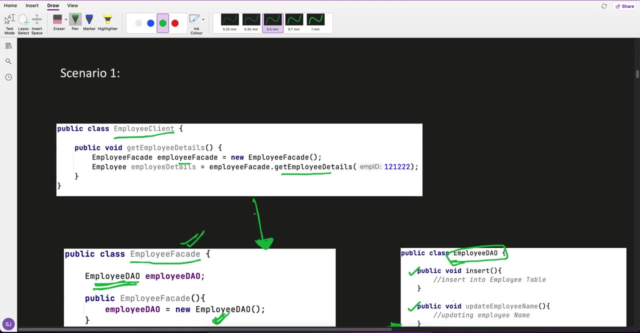 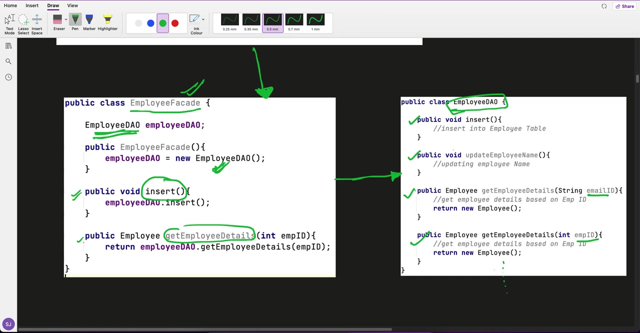 client only Wanted Insert and get employee details. so here in this client method I am just getting the employee detail. so in client has employee facade, so this has so right. so you got the scenario one. what is the scenario one? scenario one is: we can use facade when we have to just 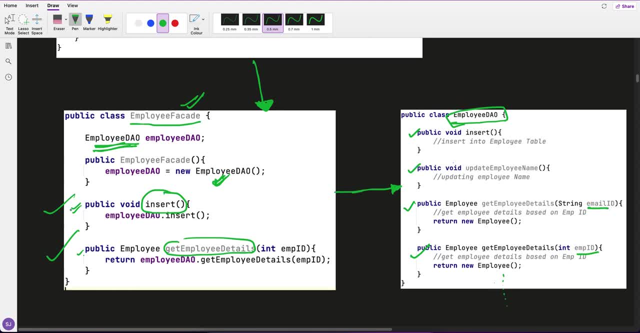 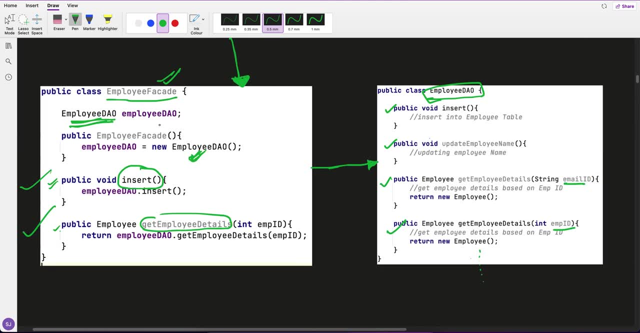 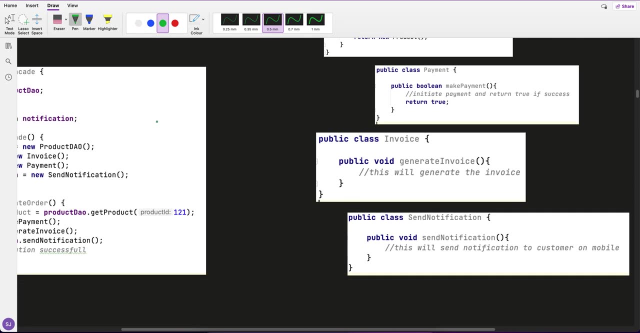 expose certain methods to the client and even if there are hundred of method and if client is not bothered in the facade, we can ignore it, okay. so this is one scenario where we can use facade. let's go to the second scenario. so in the second scenario let's say this is: 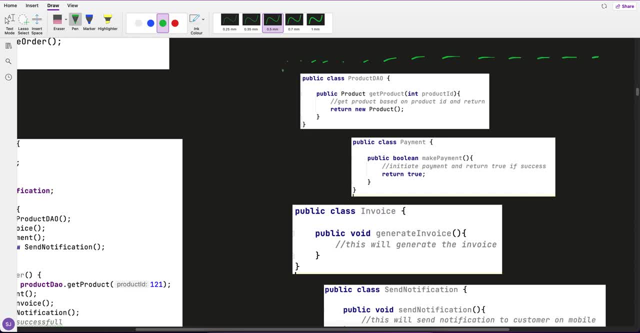 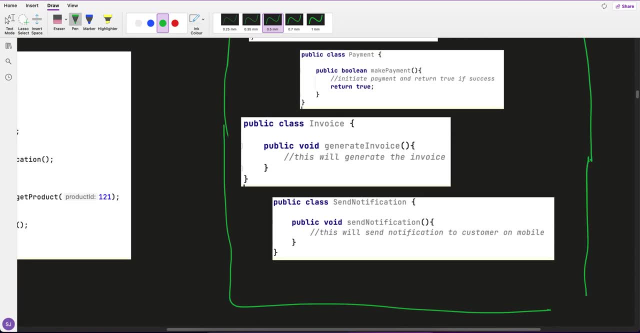 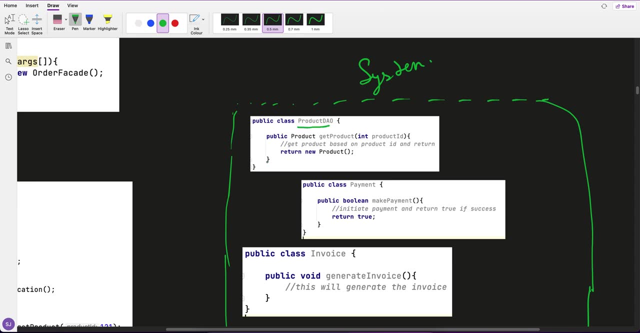 our system. let's say this is our system and it's a, let's say, complex system. this is my system. so in system I have product Dow. So product now means it will interact with product table, internally product DB, and get the product, insert product or something. so I have one method: get product okay. similarly, 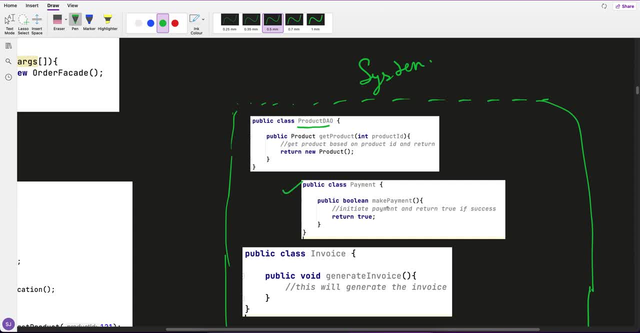 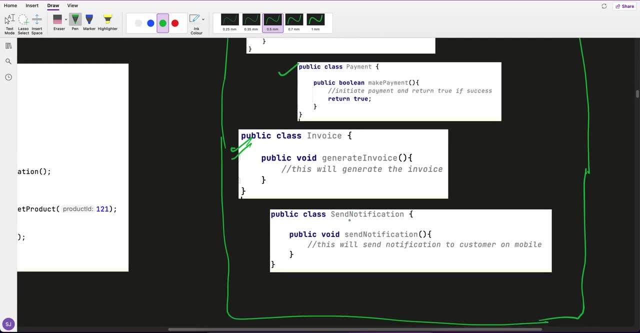 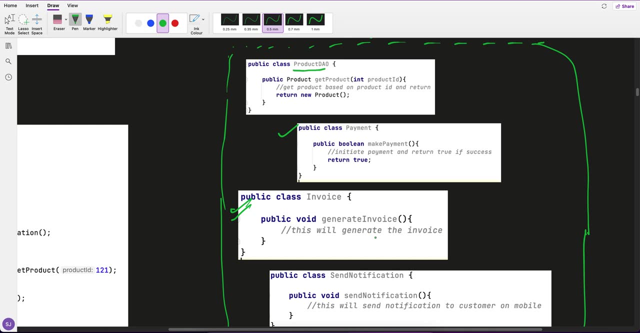 I have payment class where I have a method make payment. similarly, I have invoice where it is have a method generate invoice. similarly, I have send notification send. so just see that we have Multiple Classes, right? I haven't made any interaction. to make it simple, I haven't picked much, okay. 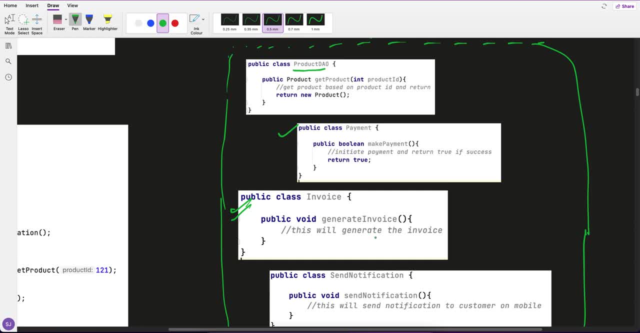 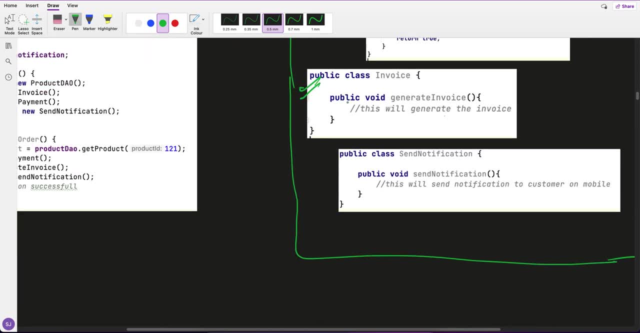 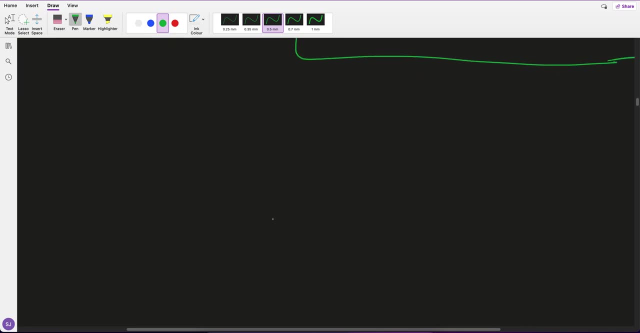 this component has his right. so there could be a complex subsystem also right, but here I just say that, okay, there are different classes present. okay, now understand this. let's take, before even telling you, the example which I have taken. let's say: I what all classes I have taken. so this is my subsystem. 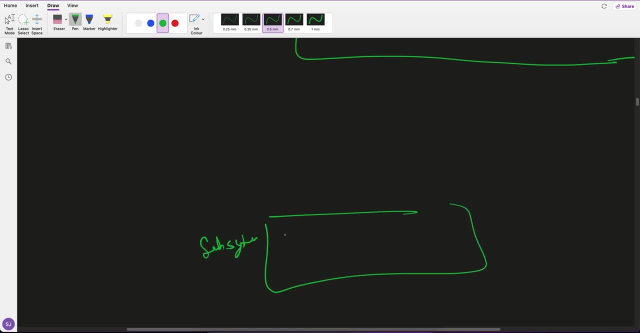 This is my subsystem. In subsystem I have Payment Product Invoice Notification Classes. Right now, let's say, if I want to make a client Right and client want to make an order, So so the purpose is to create an order. create an order, so what client will do? 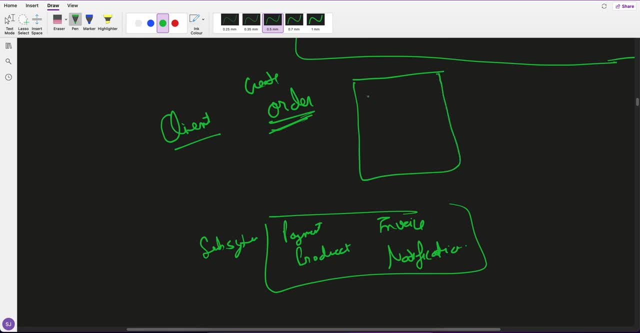 So let's say the process of creating an order is: first, get product, get product. second is make payment. make payment. third is generate invoice, generate invoice. and fourth is send notification, send notification. So when all the four steps is done, order is completed. 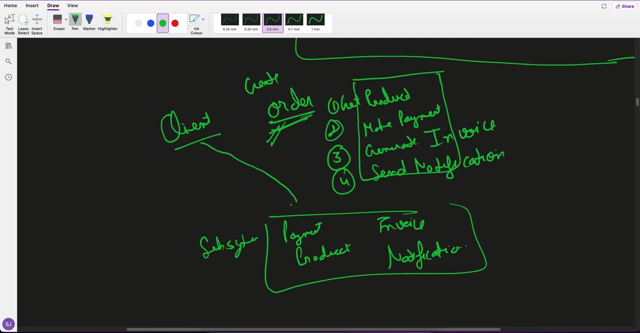 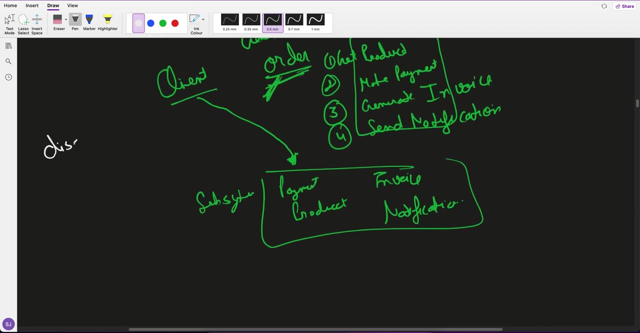 So one way is that client should have the knowledge of all this, that okay, to create an order, I need all this functionality. So here, what is the disadvantage? So disadvantage is first, if we have this, if client directly knows about, okay, so let's say in future: 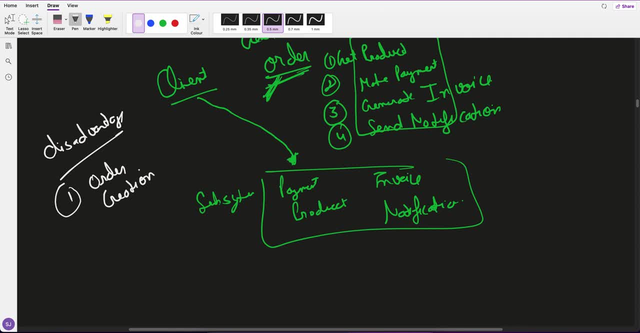 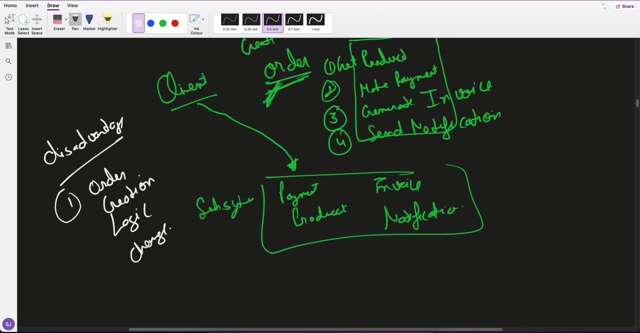 Order creation logic change. let's say I have one more thing- make payment- and I have one more step created, let's say new step for order creation. let's say one more new step added right, so client has to update Because client will break. Client has to update its order creation capability. that okay, new step has been added to create. 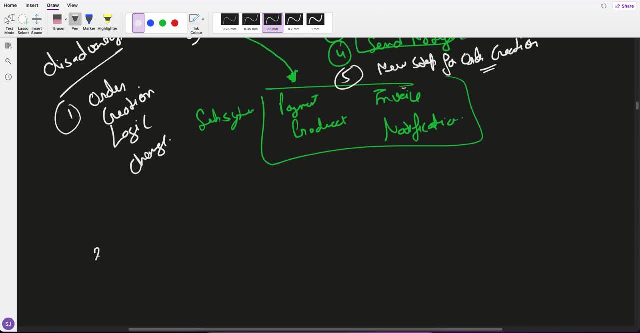 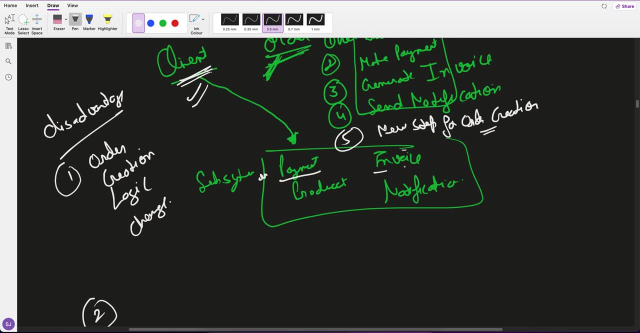 an order, So client has to change. Second, what is the problem? let's say currently payment is returning integer. or let's say invoice is returning currently boolean. Yes, invoice generated true, false right. but now let's say if any changes has been made and it's made to void. 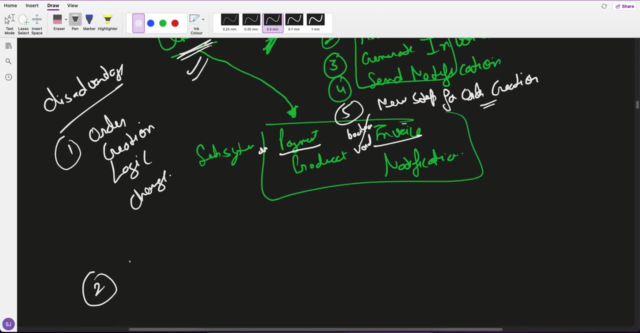 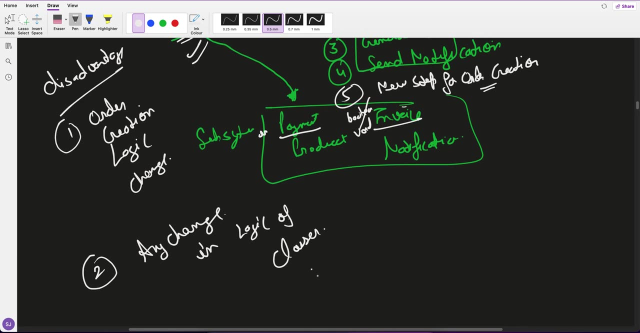 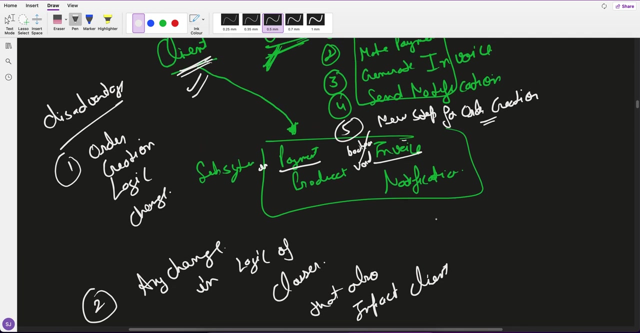 It is not returning. It is not returning anything now, right. so any change in logic of this classes that will also impact client. that also impact client. So you got the disadvantage of why client should not have this. because if in a process any new step added, 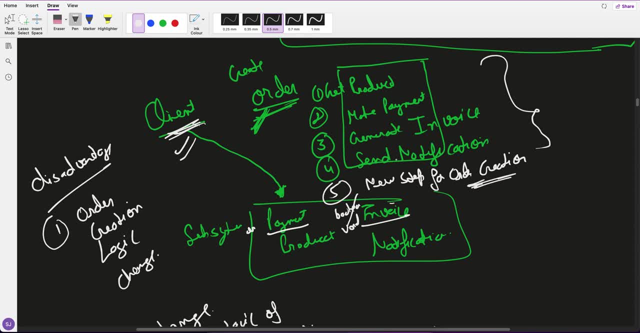 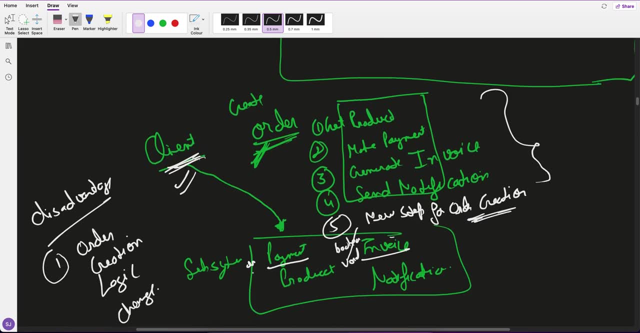 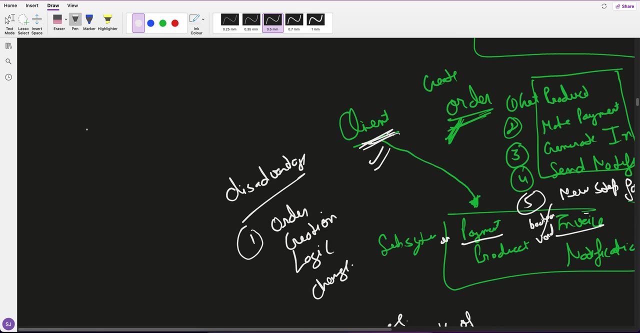 Client has to change. if in the existing steps, only if certain logic got changed, let's say return type change, then also client will get impacted. So what is the better way? So better way is bringing a facade layer, order facade layer. so all this logic steps logic. 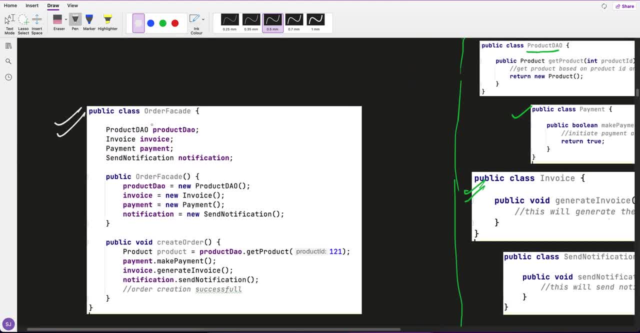 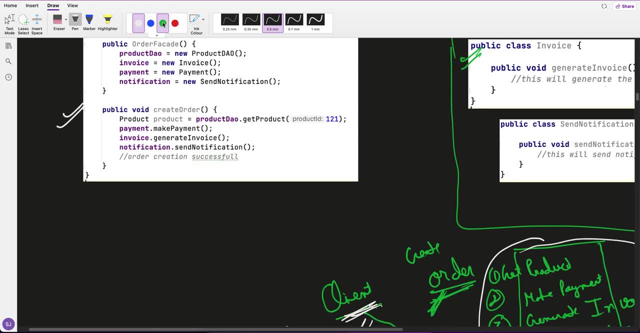 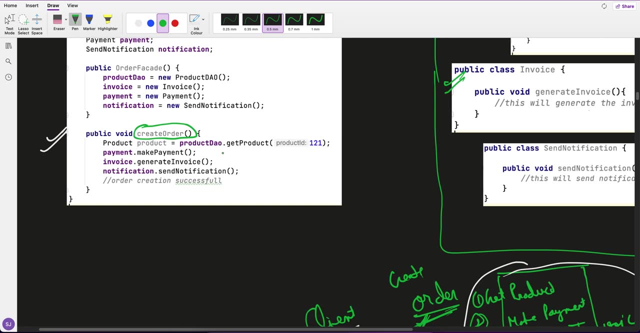 which client is keeping. we will keep at order facade layer right. so order, I have put one, create order Right. So I am saying that, hey, create an order method. I expose, and inside that I am: first fetching the product, first step. second, making a payment. third, invoice generated and then send notification. 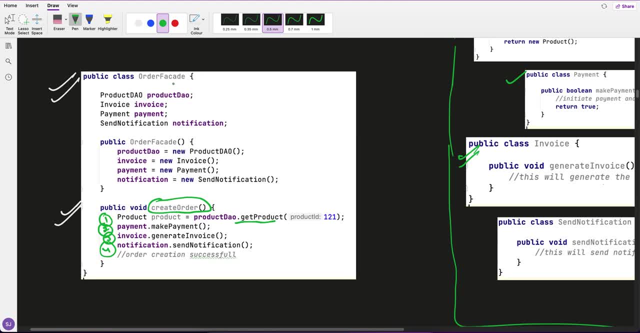 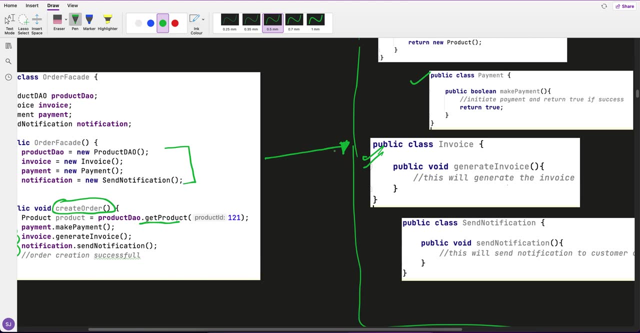 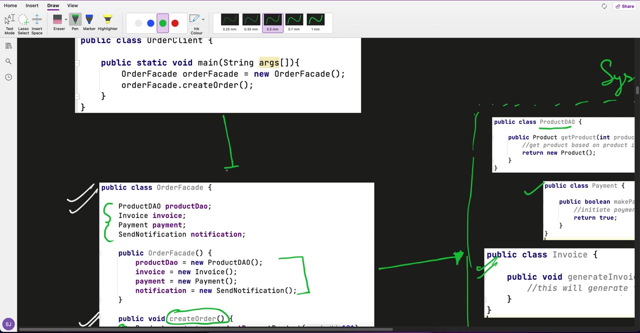 right order created successfully. So order facade has all this classes information. So it takes The responsibility of creating a object for that. so order facade has Right and now client is free. client only will call the create order of the facade. it has this one. 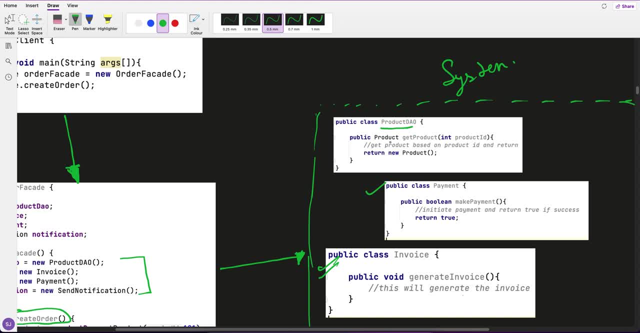 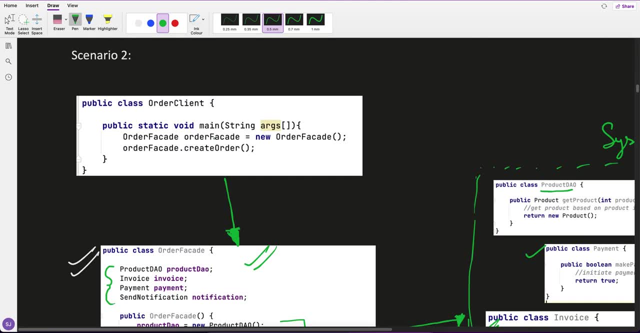 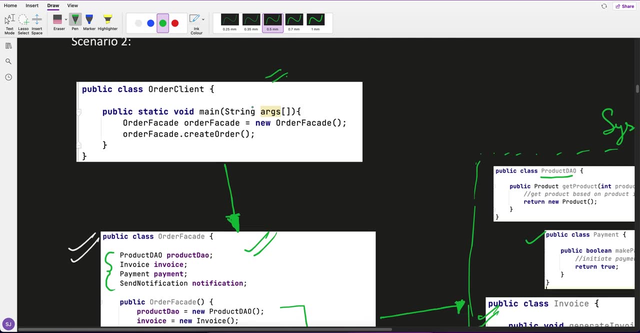 So any change in the product in the system- right, it only impact facade right, it will not impact the client. Right, Right, Right, Right, Right. So now this is the whole idea. I have been talking about all this logic and all. 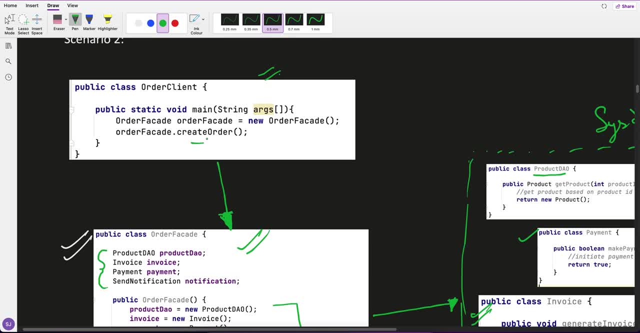 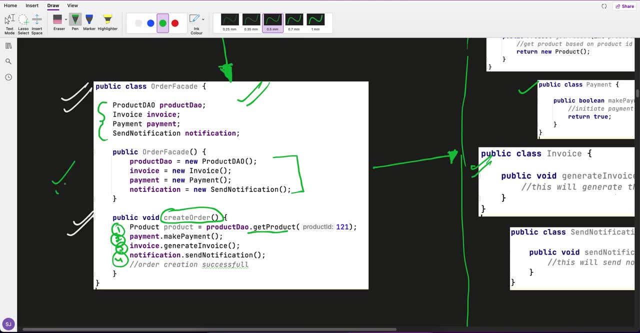 Right. So client should be like: okay, if I call this, it should happen like car. If I press this, speed should increase. if anything internally change, I don't care, Right. So that's why this is very important. You got this Okay. 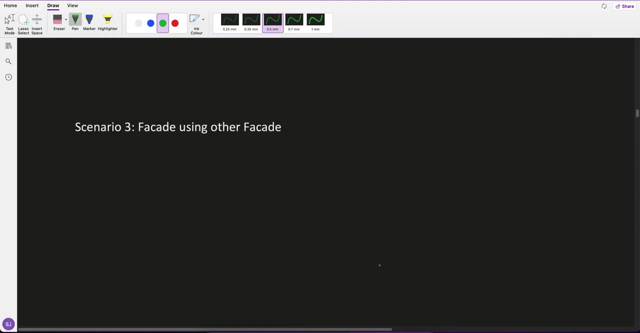 So now one more thing I want to tell you. another is facade using other facade. This is all very simple. Right till now, what we have studied is: client is calling facade and out of our. so this is our system. this is our system, which has many classes. they might be interacting with each other. 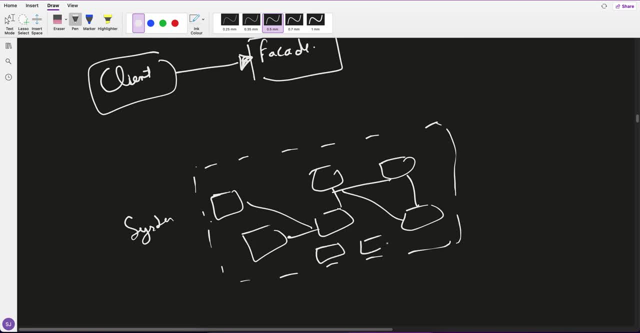 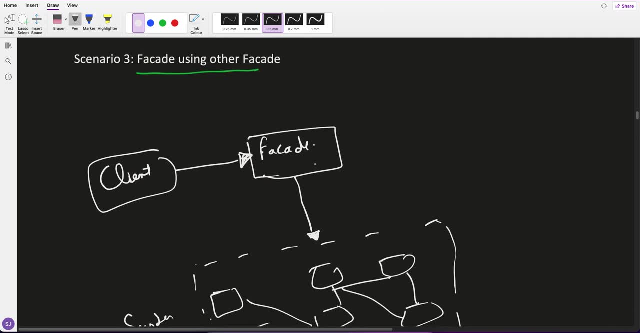 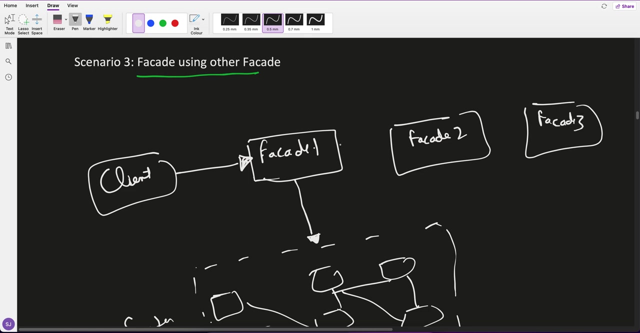 we don't know, or many classes which might not even be interacting. so currently facade can interact with them, right, as we saw. but we can also have other facade. so this is facade one. there can be a facade two, there can be a facade three. so let's say, facade one is. 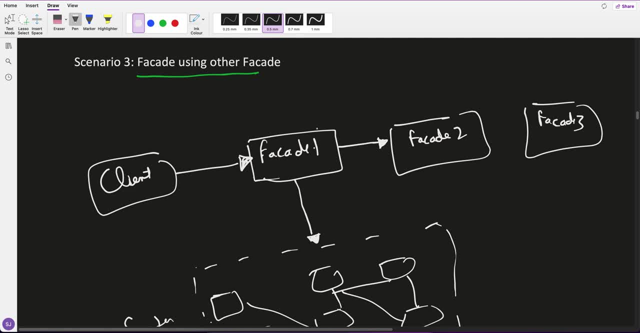 using facade two right, And facade one can also be a facade two And facade one can also be using facade three, also right. it is possible. so it can take or leverage the different facades available right. so that is also a capability which makes it facade design pattern much more powerful and easy to use. so now here, if you say that for 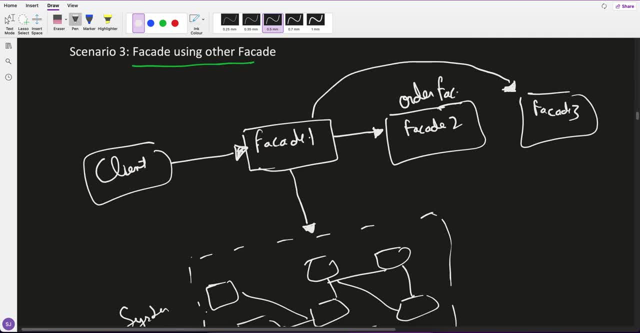 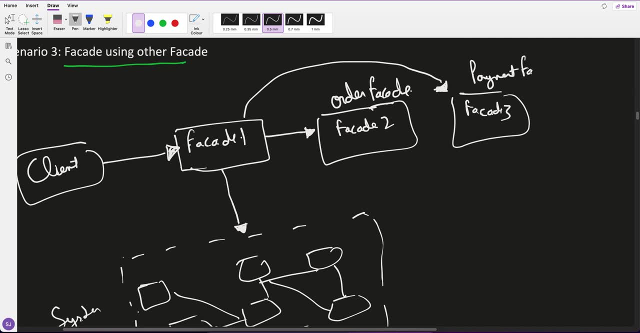 example, here I already have ordered facade right. And let's say I have a payment facade, for example, because let's say if to make a payment there would be, I think, 10 or 15 step, so we don't care, we just have created a facade. make payment, payment should be happened right. and now let's say: here is what should be that order. we have order, we have payment. and let's say: here we have a checkout facade. let's say I'm just taking an example right, just to explain checkout facade. 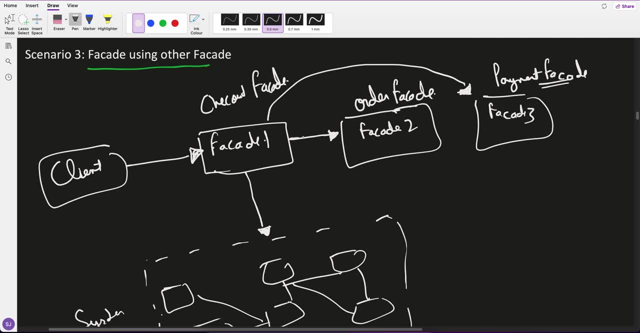 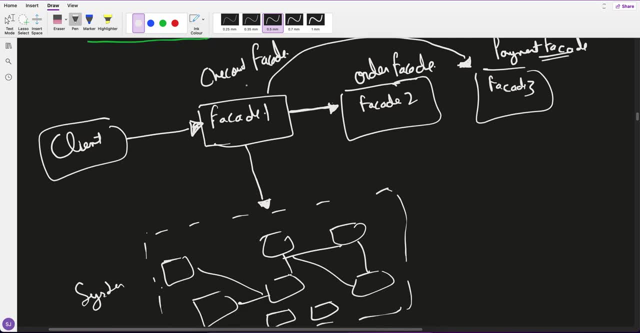 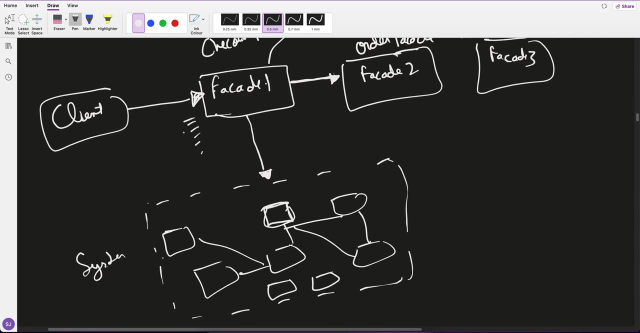 So in the checkout facade we can have is: first it will create an order and then make a payment, then checkout will get completed. and also, if it checkout facade need any other methods or any other classes, it can also call that and use it so it can create its own sequence. right, so you got it. so facade can also use another facade also. 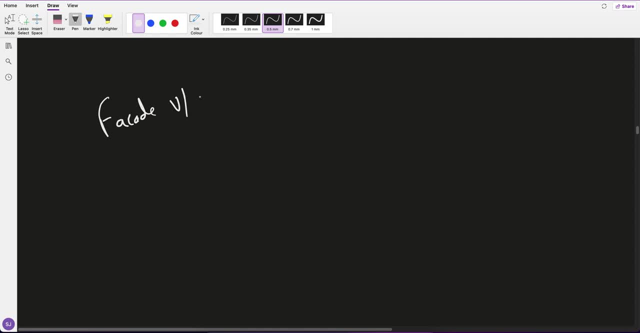 Facade versus proxy. Now you can ask me, hey shash, how the facade and proxy are different. so if you remember in proxy what we have done, let's say we have employee dow. so here this is. let's say, in proxy, we have created an interface, this is an interface and this is the real object. 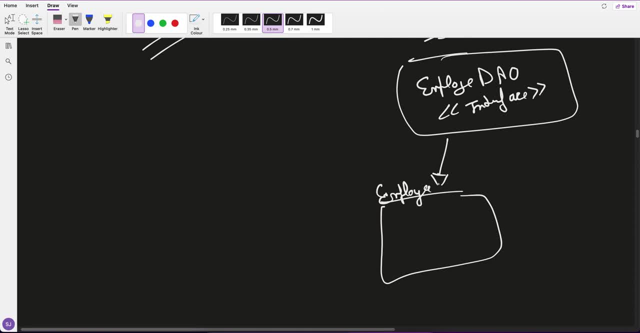 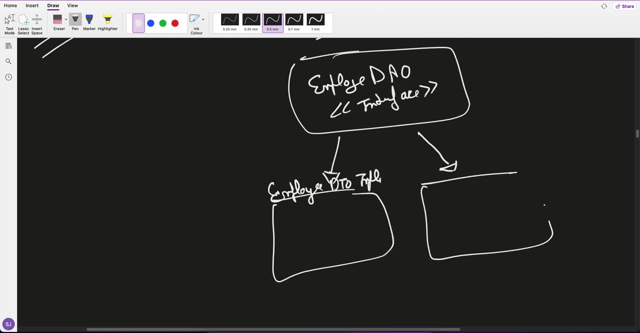 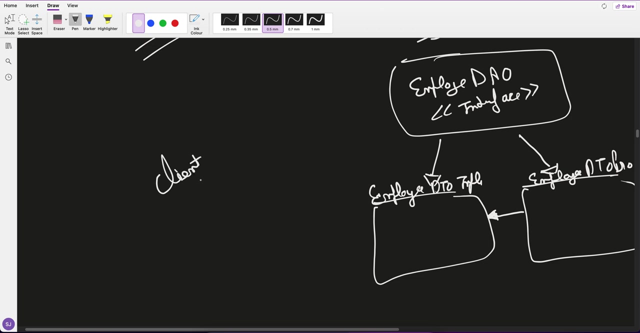 Employee: DT, DT, DT, DT, DT, DT, DTO, IMPL, implementation. so in proxy we create one proxy here, employee DTO proxy and proxy internally calls this IMPL, so client calls proxy, so client call proxy and proxy actually calls the actual object. right. so 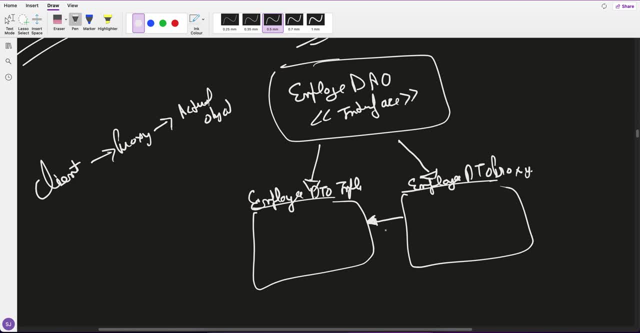 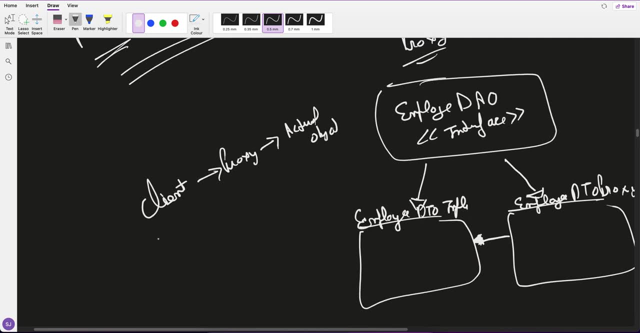 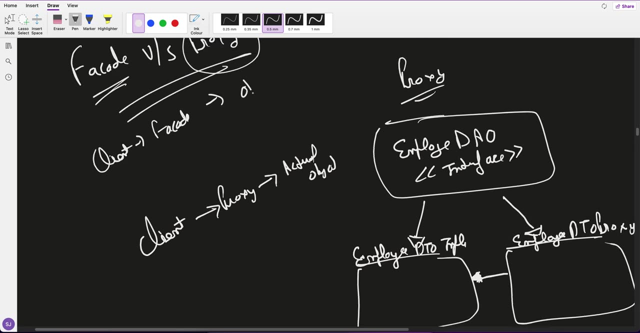 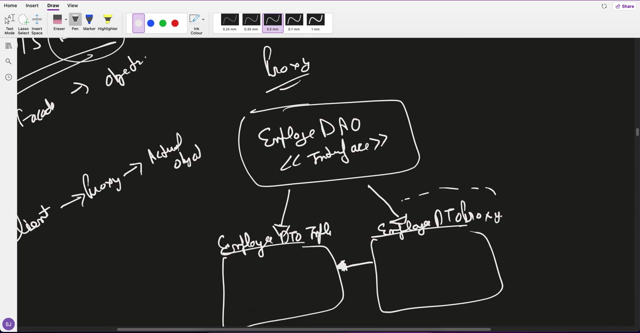 client calling Employee- DTO proxy and employee DTO proxy is calling the this one. So now you can say that, hey, it is very much similar to facade Here now in facade Client is calling facade And facade is calling the actual objects Right, so you can see how they are different from differences if you see the proxy. 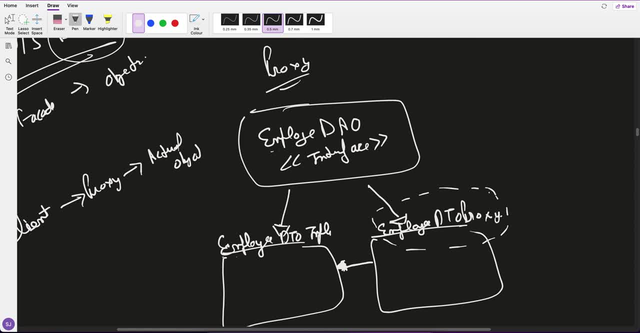 Proxy is for a particular object. so let's say say this object, so whatever the interface of this class, proxy is also of the same interface, right? so this is of the same interface and proxy takes care of a particular object. so now here inside it's a employee DTO, right? so proxy will take care of this, only proxy. 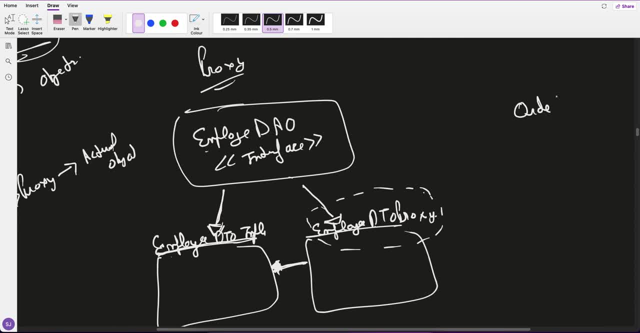 let's say, if there are another DTO- let's say order DTO proxy- this proxy will not take care of this one right, so a proxy can take care of only so. this is wrong. a proxy can take care of only one object, right, and the type of this proxy is also same as that object. 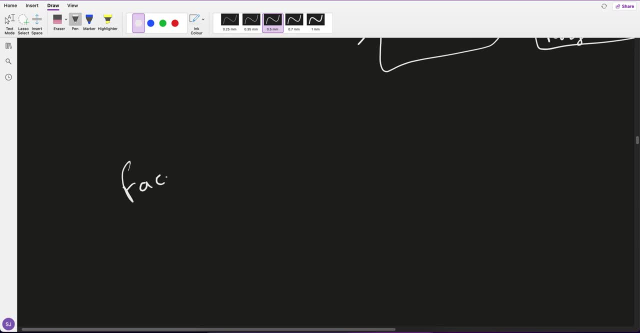 which it is taking care of now. see facade versus adapter. so in adapter, you know, right, we have an actual interface, right? or you can say that original interface, right. so let's say I have taken an example of, let's say, this socket, so this is an original interface. and then you have a client, so let's say your. 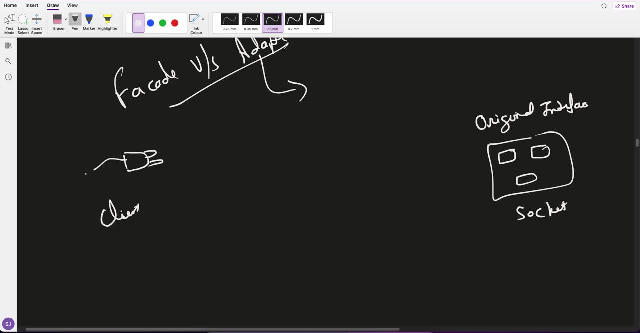 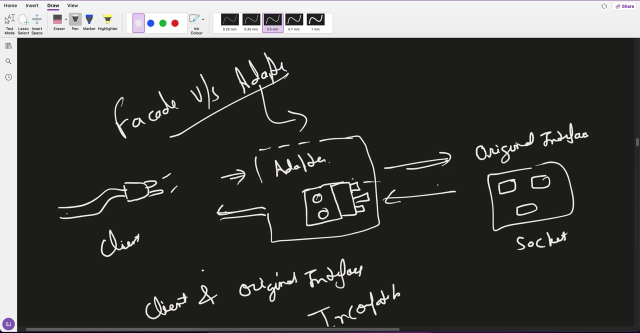 client is this right. so they are currently incompatible. so client and your client is incompatible. You are original interface, uh, incompatible. so we create an adaptor in mid. so we create an adaptor in mid so that client can talk with adaptor, adaptor can talk with original and it can do kind of a mediator, right, so you have got. adaptor is used to bring the compatibility.